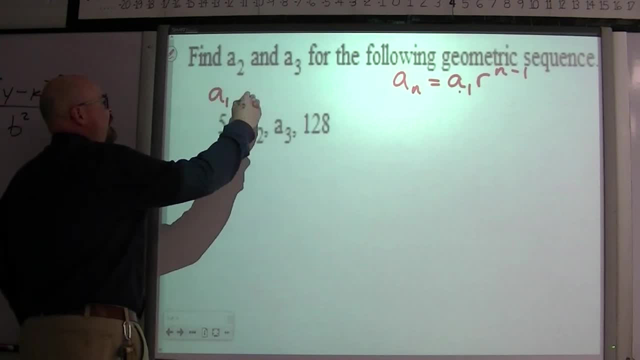 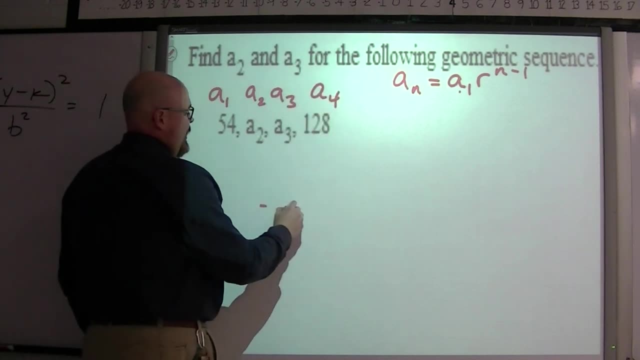 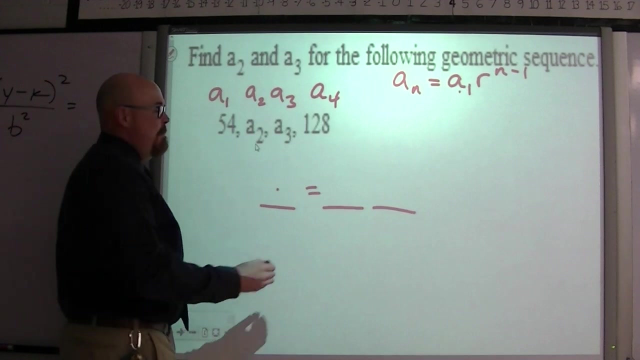 Okay. so we talked about a different situation where, if this is the first term, we've got the second term here, we've got the third term here and this is the fourth term. We talked about how I can set up, I can set up an equation where I can find any term that I want based on. 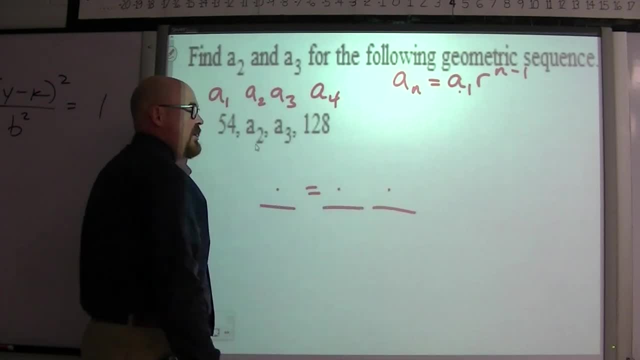 anything term that I have. if I know, the common ratio and the power that I use here and the term number here add up to be whatever term number I have here right. so, just as an example for what we're looking at right here, what do I know? I? 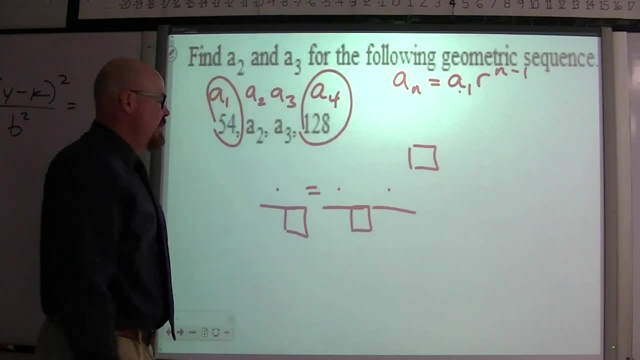 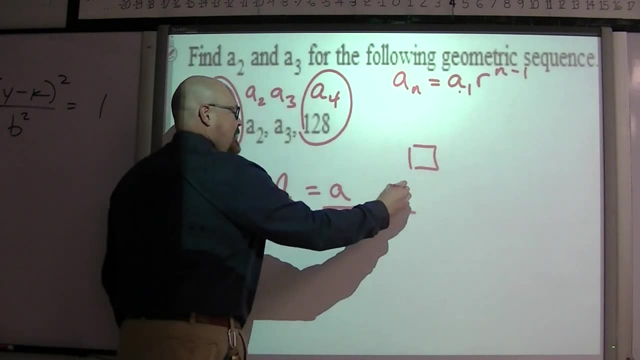 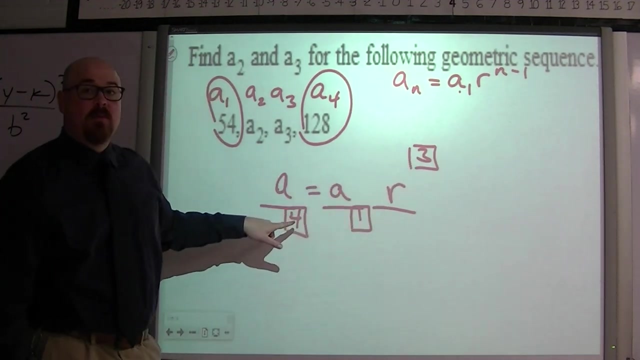 know the first term and I know the fourth term. so that means that if I know, if I know the fourth term and I know the first term, I can get that by doing by multiplying by the common ratio cube, these numbers add to be this number. so this is a situation where, because these are the only two terms that I know, this- 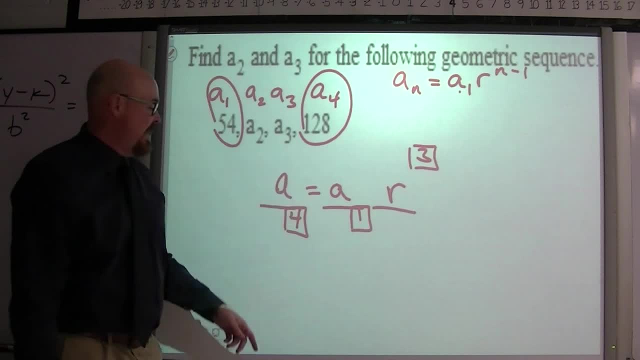 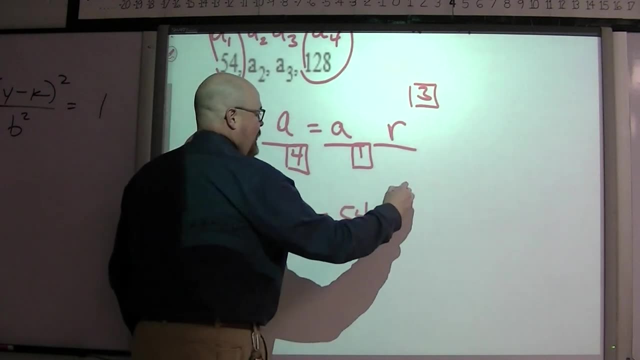 is really the only useful equation that I can set up. okay, now fill in what we know about that. the fourth term is 128, the first term is 54 and I want to know the common ratio. this is going to help me solve for the common ratio. it's the. 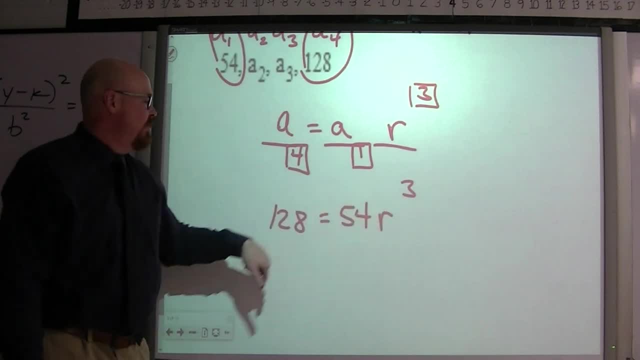 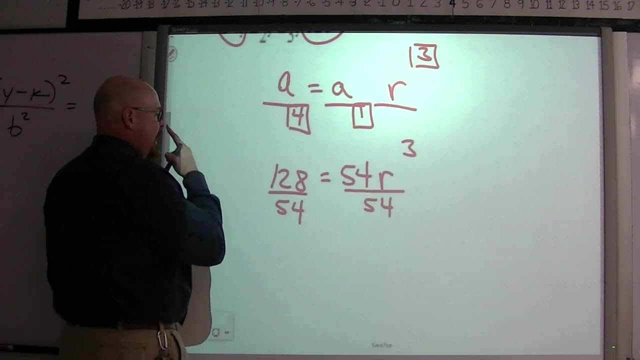 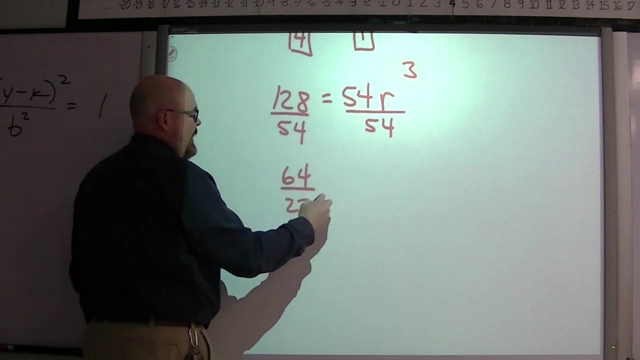 only variable in this problem now. so I can solve for R cubed: if I take the, if I divide both sides by 54 and isolate that term, 128 over 54 is 64 over 27 and I'm going to write it like that for a reason- I'm not actually trying to get a decimal for this, because 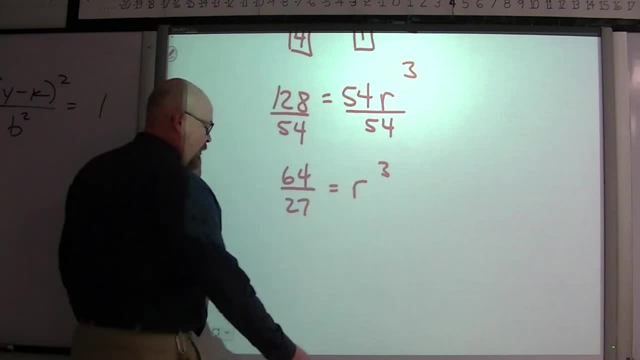 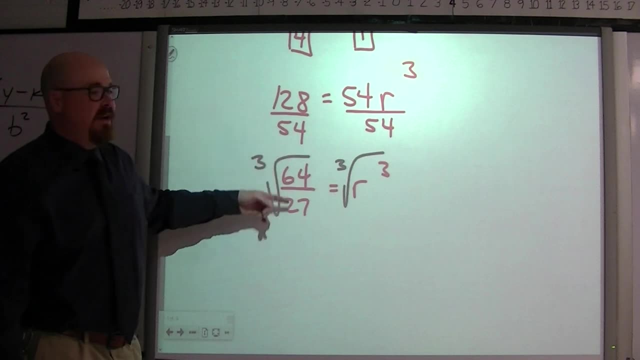 I'm not done solving yet and if I take the cube root over here, right, we take the cube root to get rid of that. I'm taking the cube root of this and the reason that I didn't write a decimal for this right away is because these are. 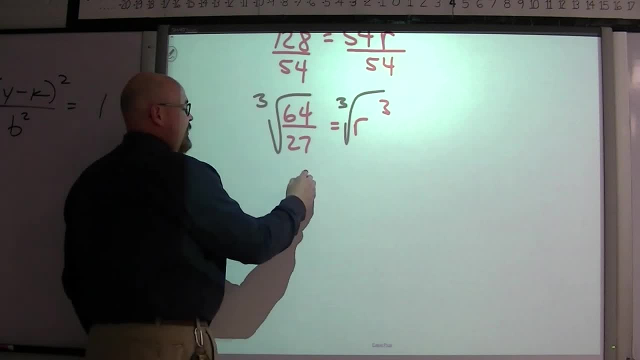 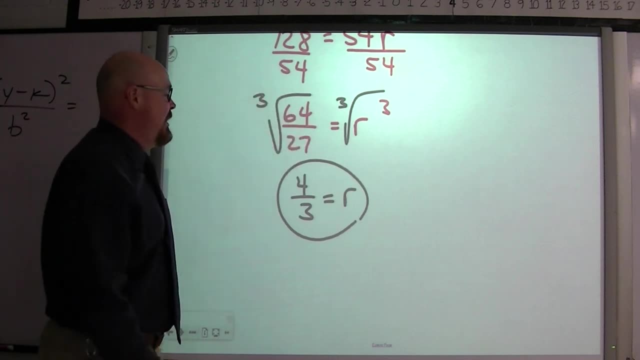 both perfect cubes. so taking the cube root of both of those is 4 over 3. now I have the common ratio right now. you could have gotten a decimal for this, taking the cube root, and it would have said: you know, 1.3, repeating, which is fine, right, but I'd